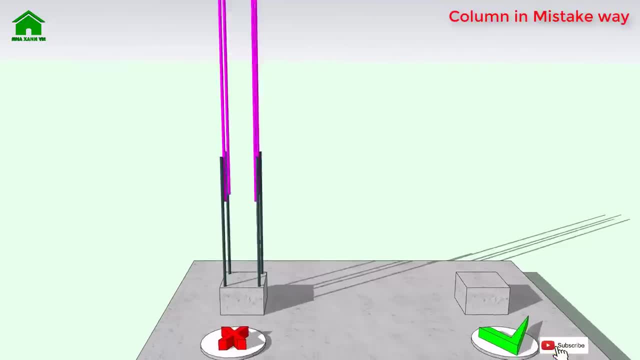 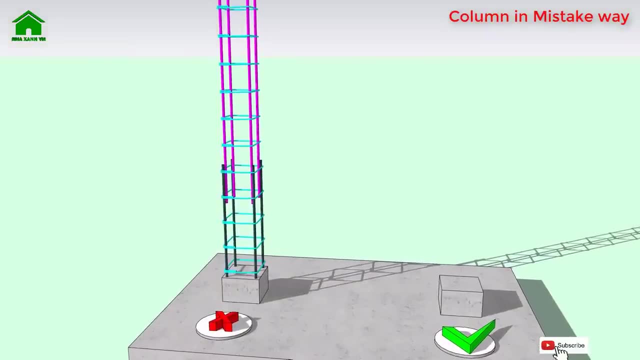 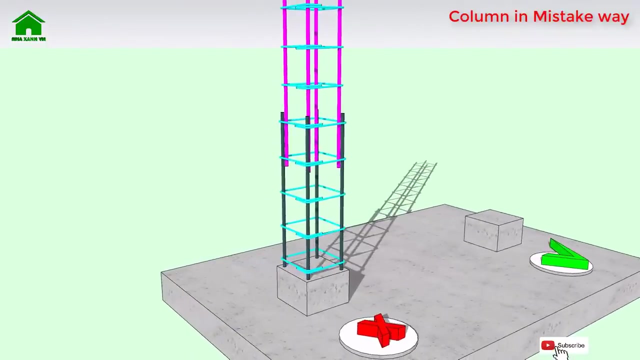 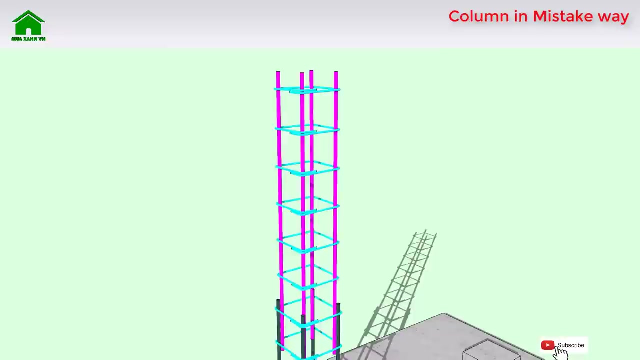 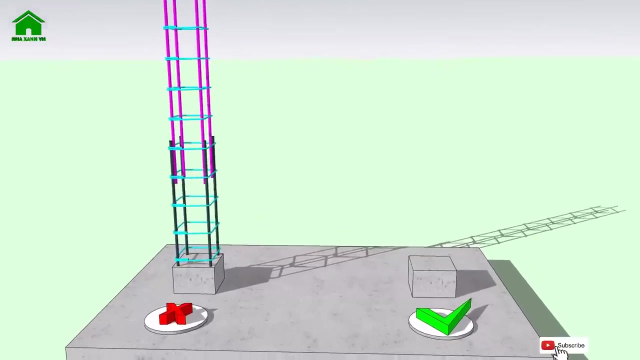 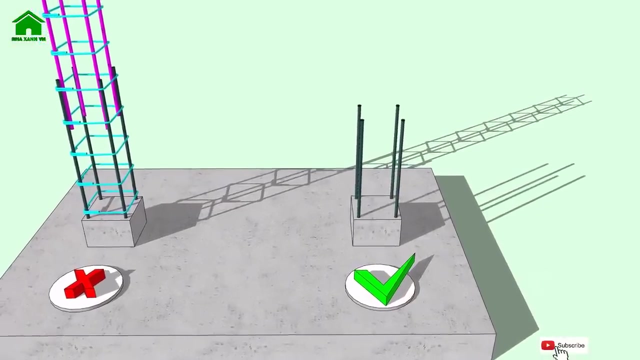 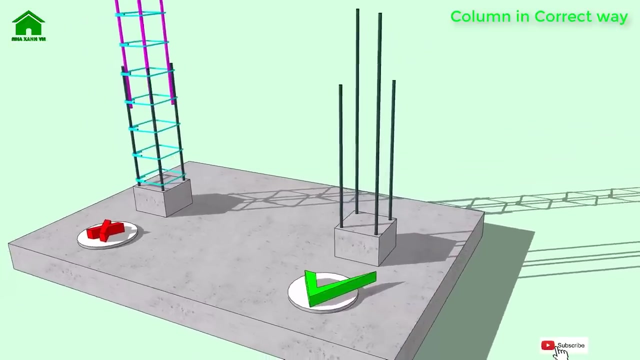 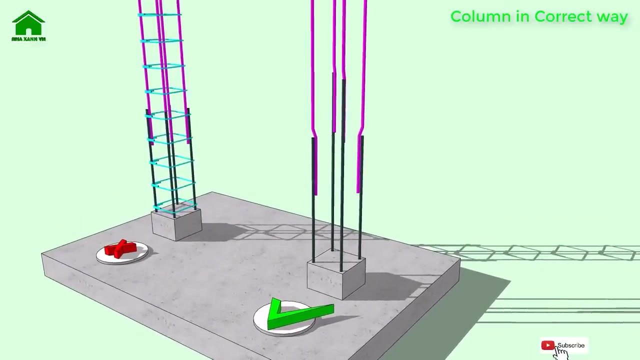 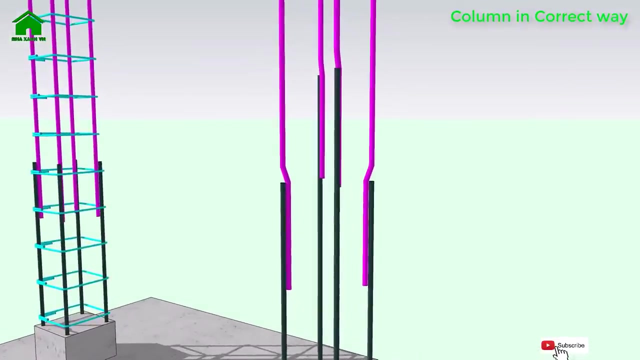 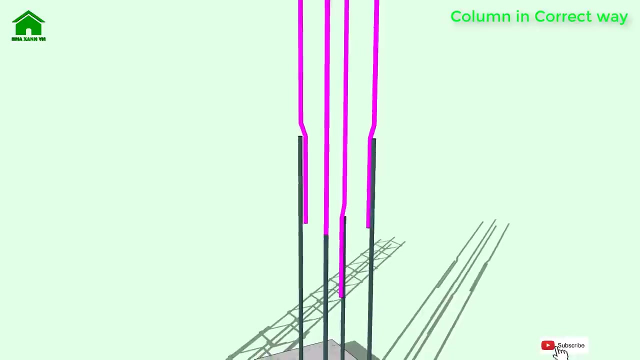 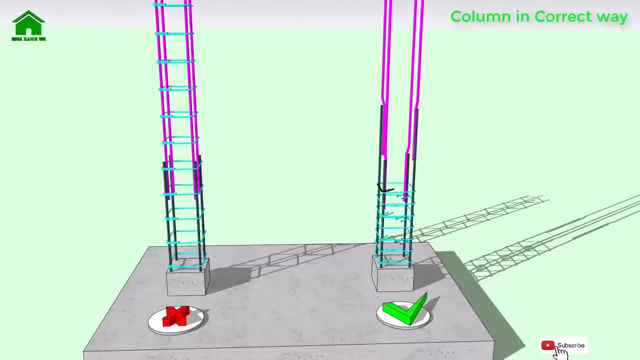 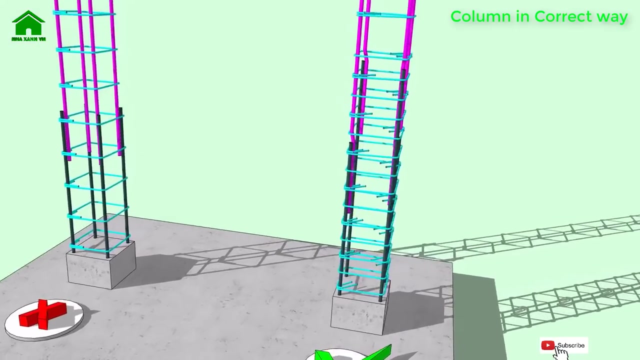 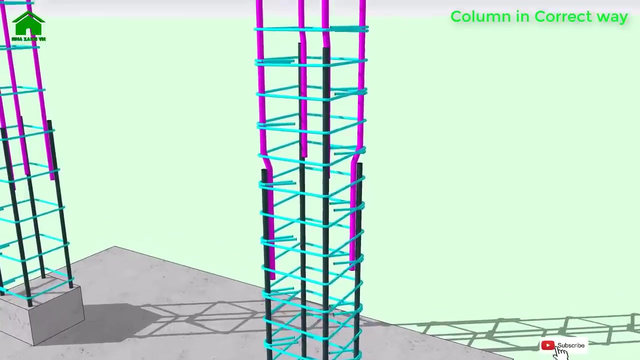 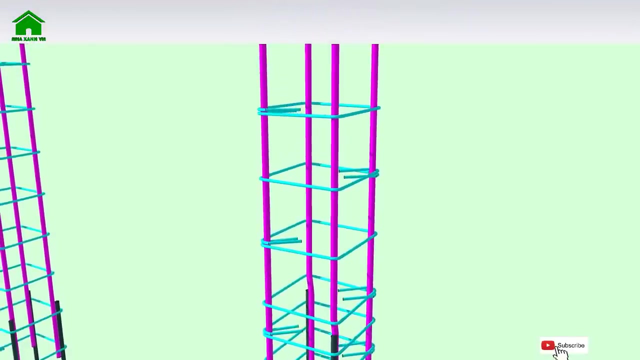 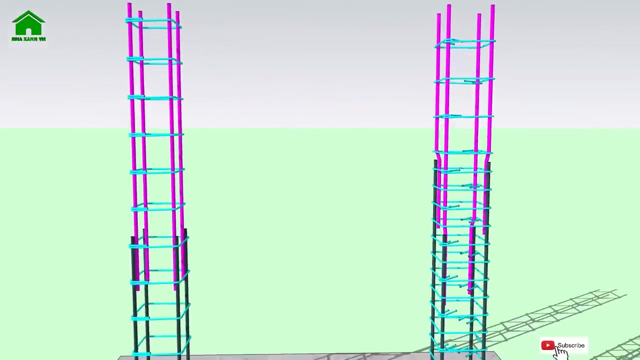 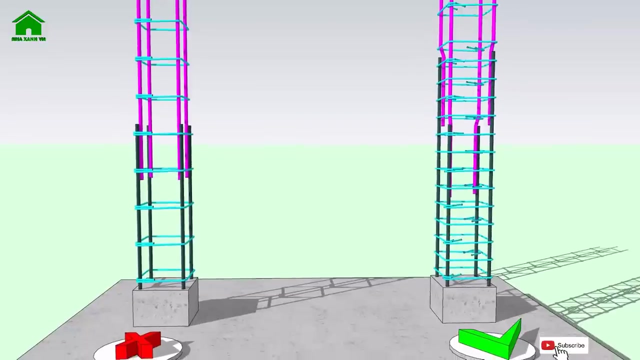 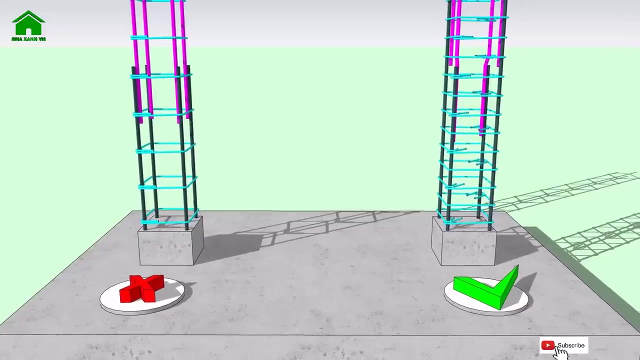 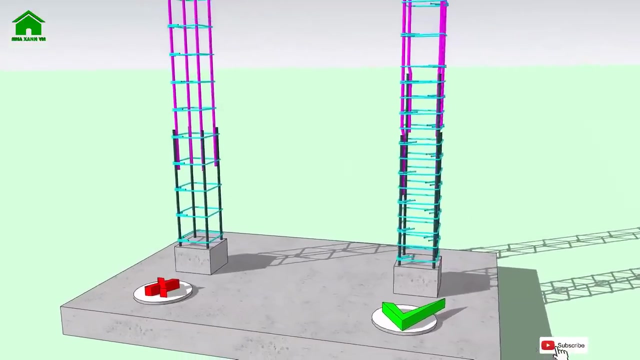 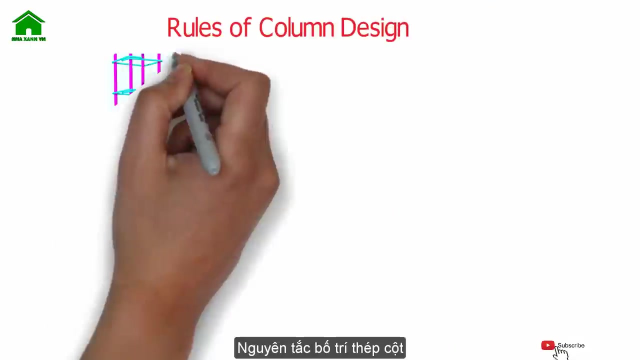 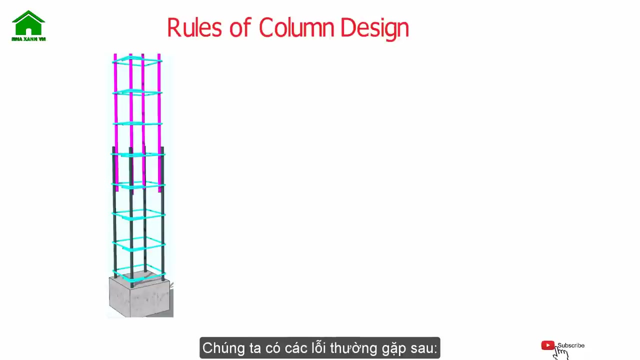 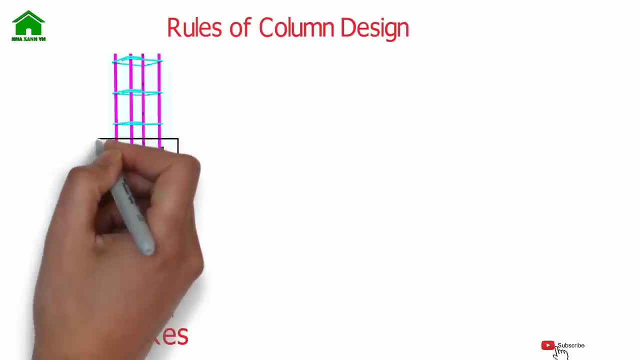 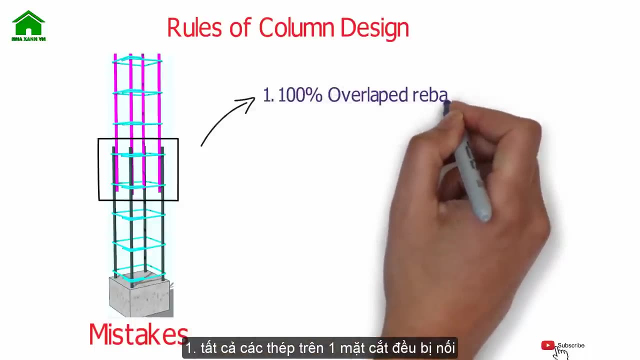 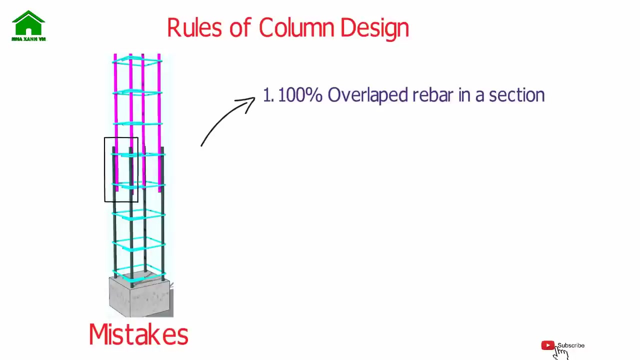 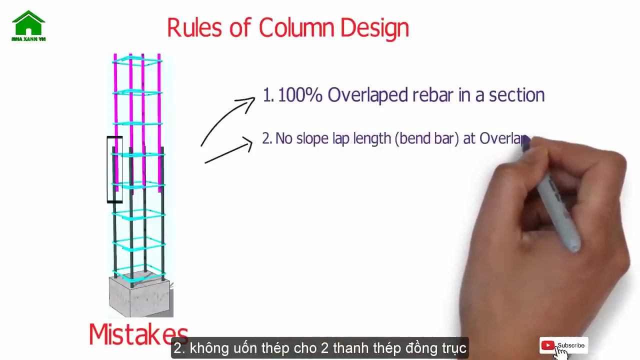 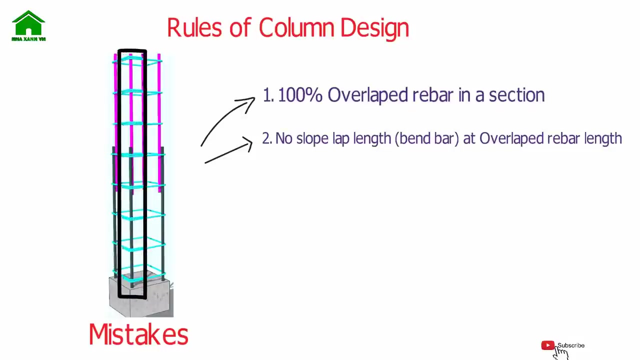 In a mixed-text way. we have some mixed-text: 1. 100% of the last rebar in a section. 2. No slop-luck length. As overlap rebar length, it means no bending bar. 3. All ties with end bend in one direction. 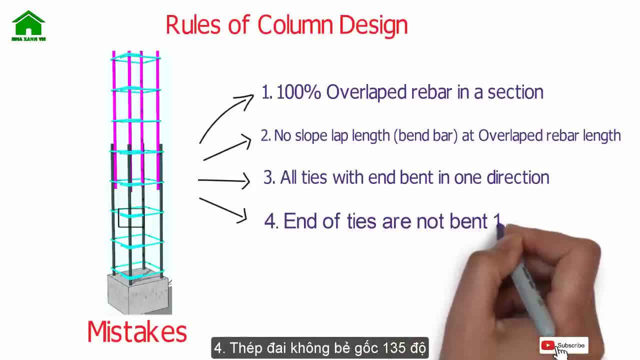 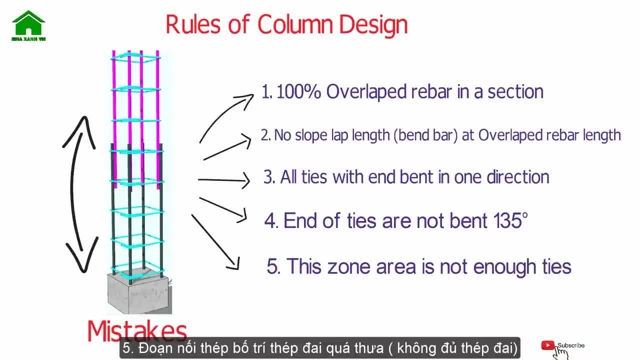 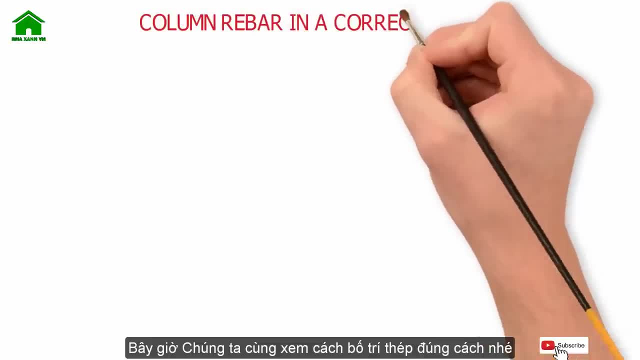 79. End of ties are not bend 135 degrees. 79. End of ties are not bend 135 degrees. This area is not enough ties. Now we are talking about the column V bar in the correct way. In the correct way, we have five rules. 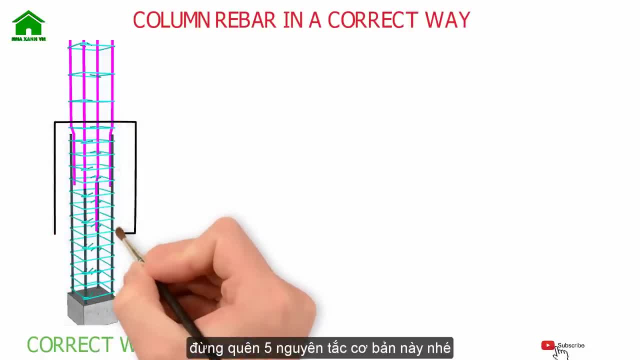 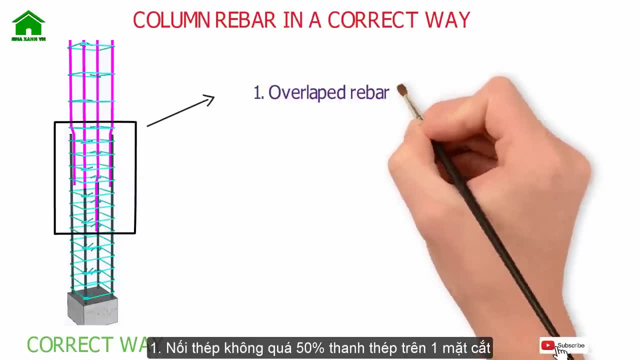 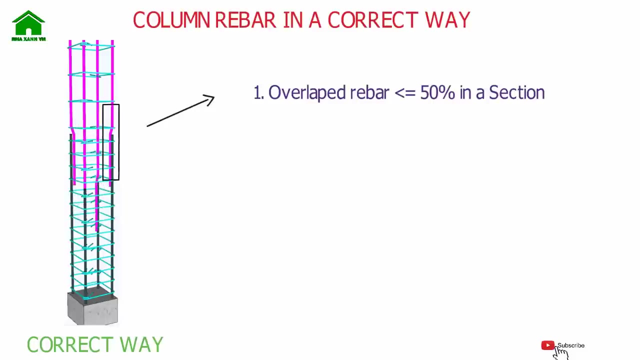 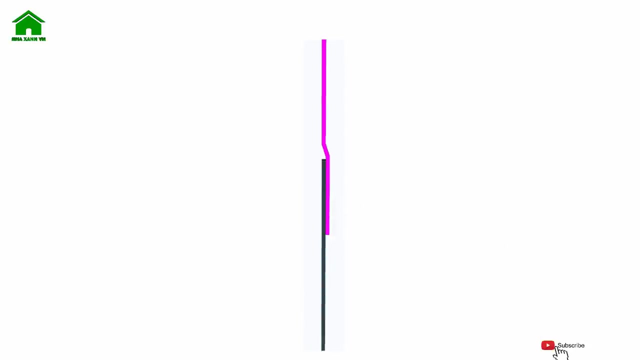 Don't forget this five rule Like this: 1. Overlocked V bar: not over 50% of the inner section. 2. Lap length with the lap 1-6.. Like this, It's a bending bar. 3. The end of ties. 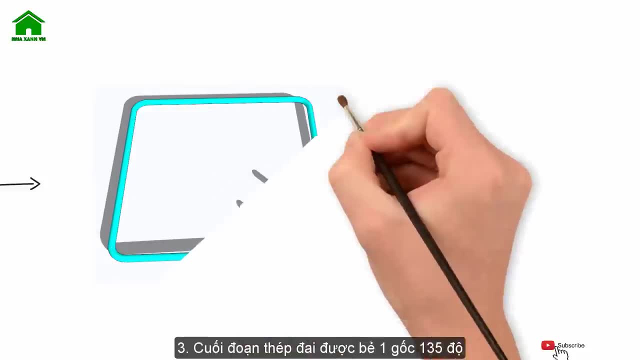 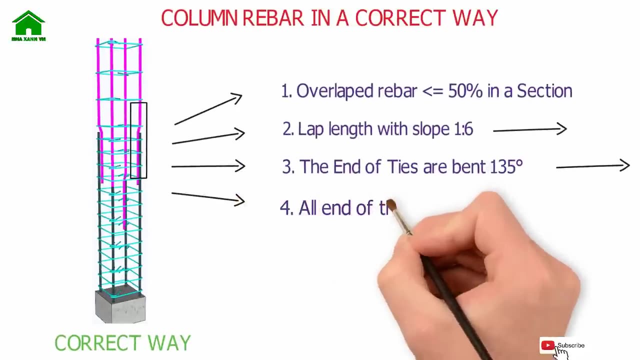 2. The end of ties. 3. The end of ties. 4. The end of ties. 5. The end of ties are bent 135 degree like this. Therefore, all anaphthites are not one direction. 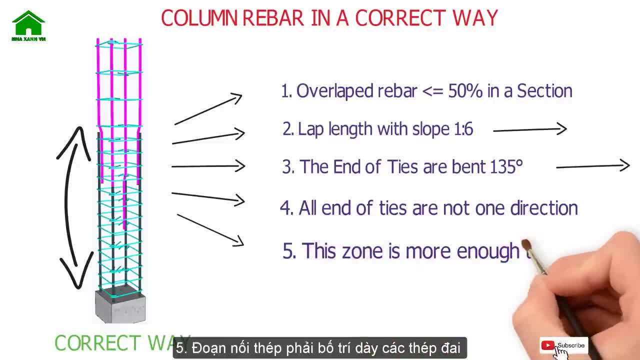 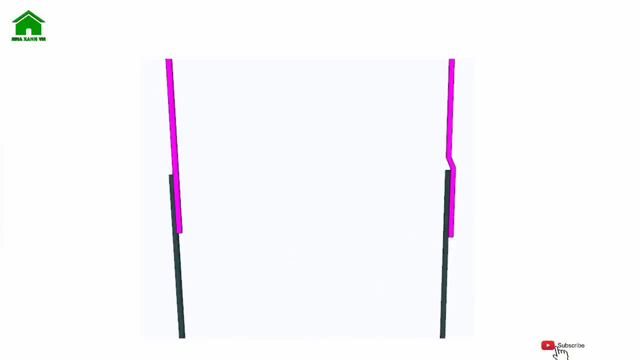 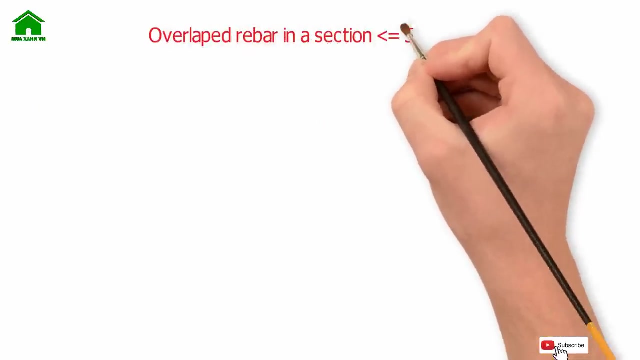 And the fifth. this zone is more inner thighs. Suddenly I feel like I can go further. The connecting position of the upper left side and the upper right side are the hip joint joints. The bony peritoneum muscle of the face does not transfer shock and irritation to the bony作od inside the 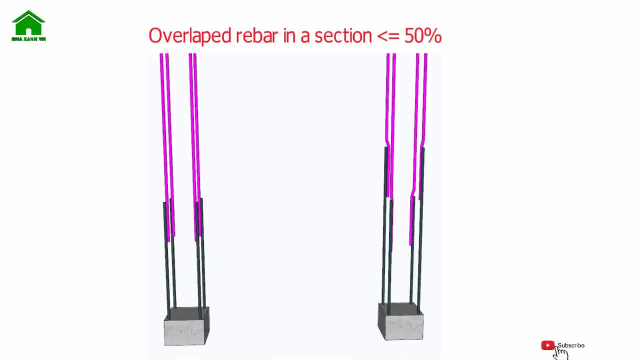 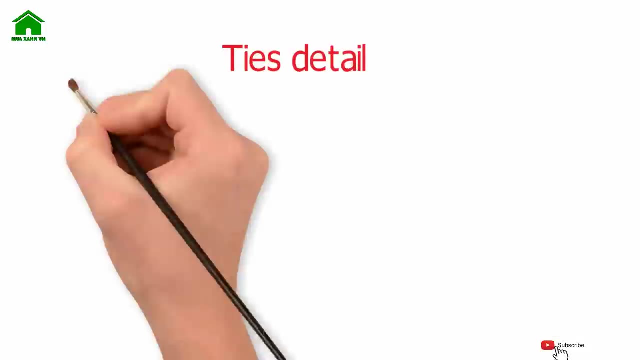 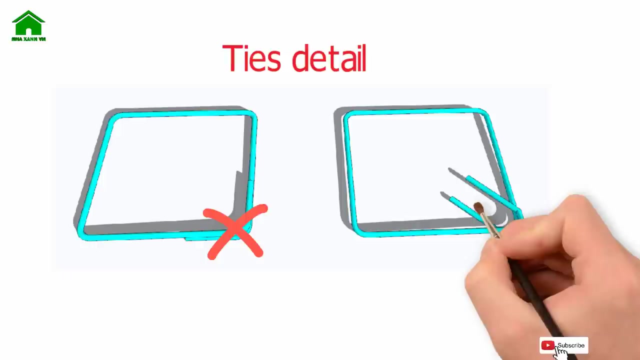 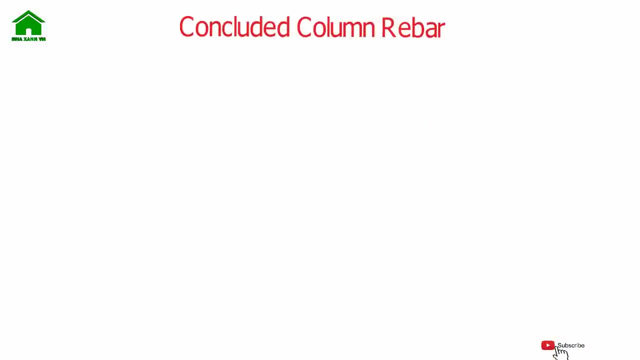 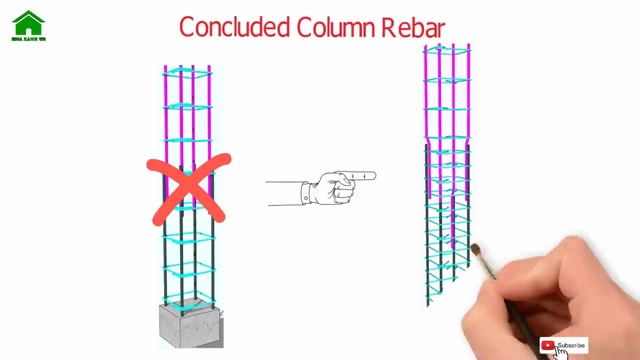 We do anyone, so It is not easy to find out the information like this, so I put a lot of effort into this. Now, this is the map that I took in the last video, so it's not that difficult to understand. Let's get right into it. Ascom.